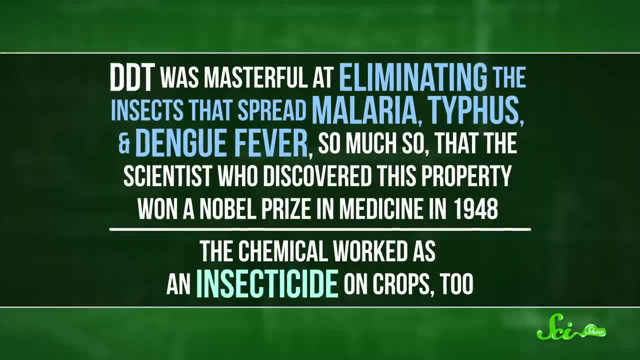 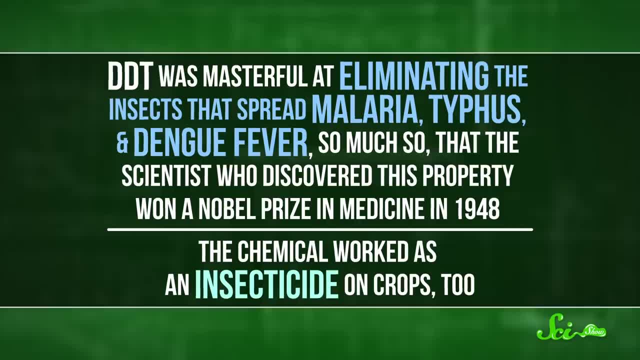 DDT was masterful at eliminating the insects that spread malaria, typhus and dengue fever, So much so that the scientists who discovered this property won a Nobel Prize in Medicine in 1948.. The chemical worked as an insecticide on crops too. 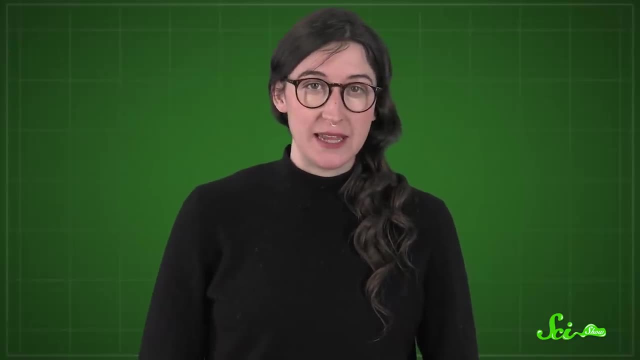 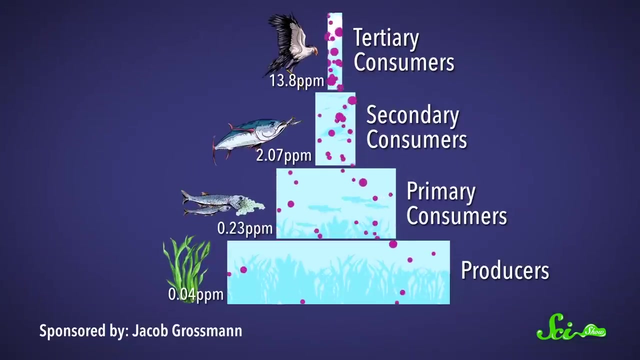 But it didn't come without cost. Although it's moderately safe for humans to handle, in low doses, DDT builds up or bioaccumulates in the fat tissues of exposed animals And, because the pesticide degrades so slowly in the environment, it moves up the food chain. 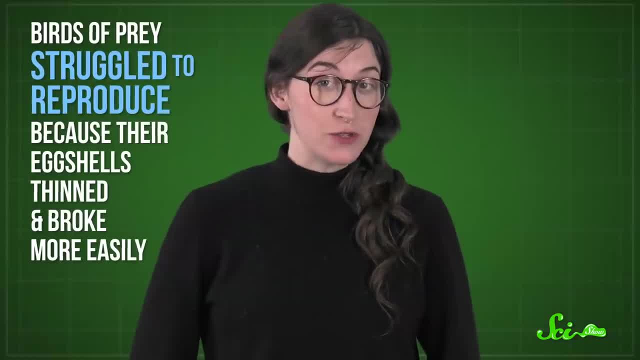 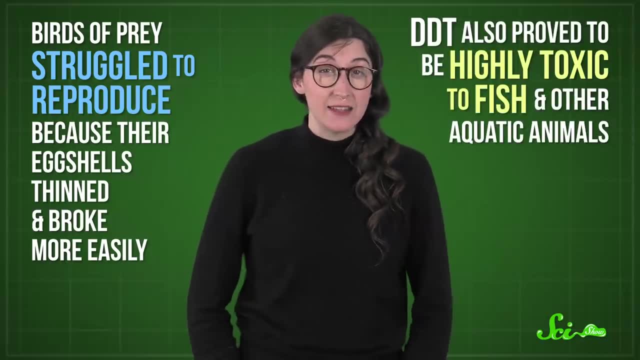 in a process called biomagnification. As a result, birds of prey struggled to reproduce because their eggshells thinned and broke more easily. DDT also proved to be highly toxic to fish and other aquatic animals. Basically, it's not good for ecosystems. 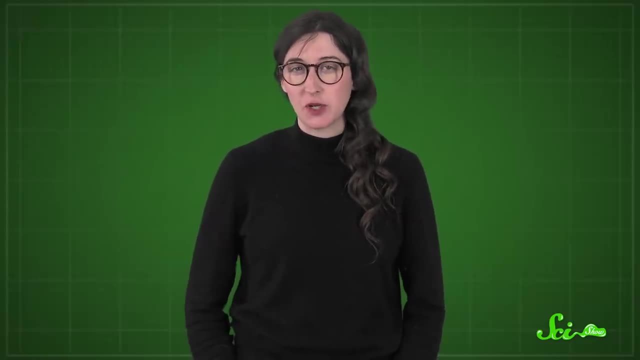 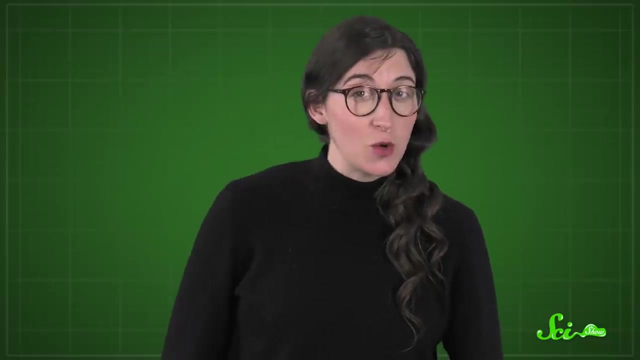 In 1962, Rachel Carson famously sounded the alarm in her book Silent Spring, and a decade later the US government did it: It banned DDT for agricultural use. In its own way, though, DDT helped to spark the modern environmental movement. 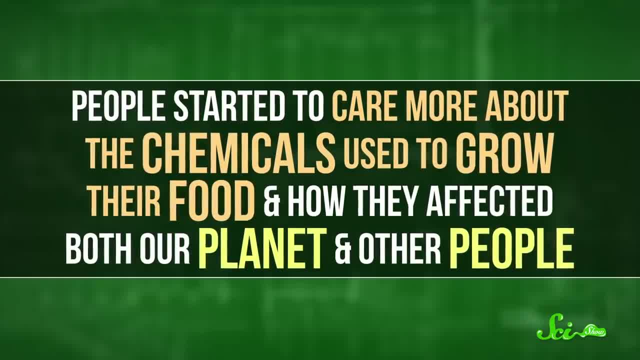 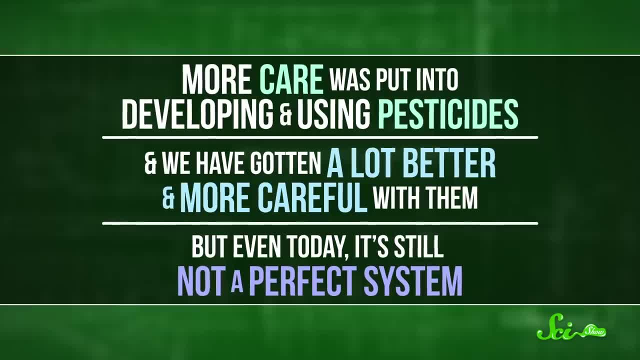 People started to care more about the chemicals used to grow their food and how they affected both our planet and other people. More care was put into developing and using pesticides, And we have gotten a lot better and more careful with them, But even today, it's still not a perfect system. 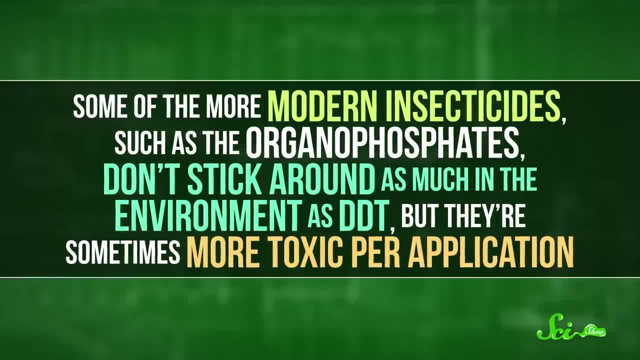 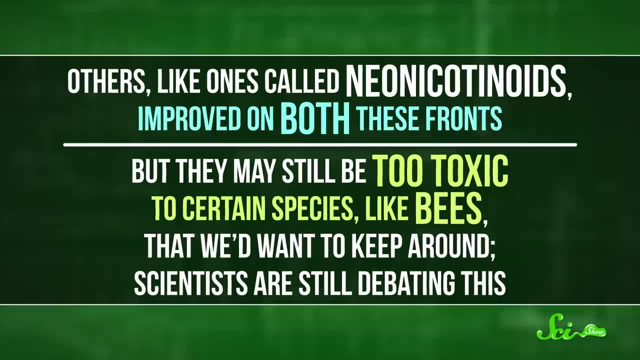 Some of the more modern insecticides, such as the organophosphates, don't stick around as much in the environment as DDT, But they're sometimes more toxic per application. Others, like ones called neonicotinoids, improved on both these fronts. 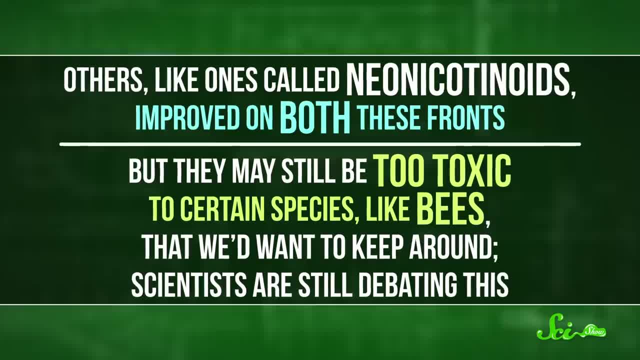 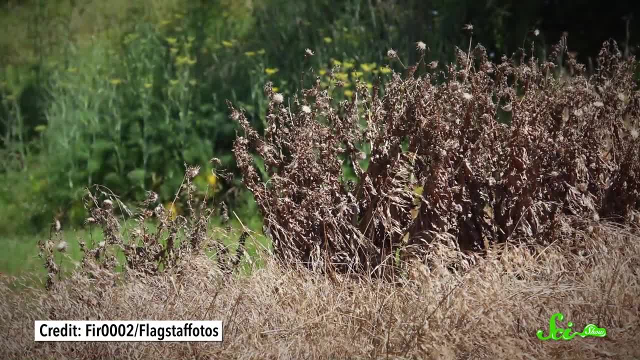 But they may still be too toxic to certain species, like bees, that we'd want to keep around. Scientists are still debating this. Herbicides also have their problems. While insecticides tend to interfere with the nervous system of insects, herbicides attack weeds by preventing them from growing. 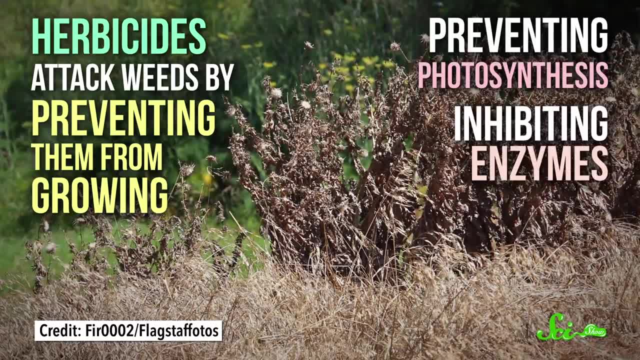 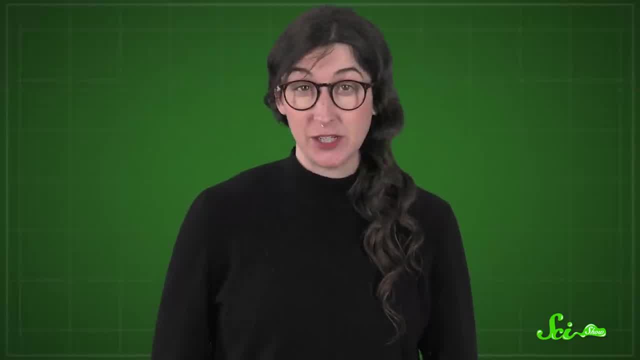 Often, they do this by preventing photosynthesis or by inhibiting enzymes that plants use to make new cell walls: amino acids and other chemicals. Unfortunately, under certain conditions and concentrations, some of these are so acutely toxic to humans that people have used them to commit suicide. Others are less dangerous to people and some other animals, but they can still leach into groundwater, where they can harm fish. And even though we're making progress, other types of pesticides have their own struggles too. Really, none of these are ideal. It'd be great if we didn't have to use them, and there are strategies people can use to reduce use, But when you run into a big problem like a massive cockroach infestation in your kitchen, you'll be glad they exist. 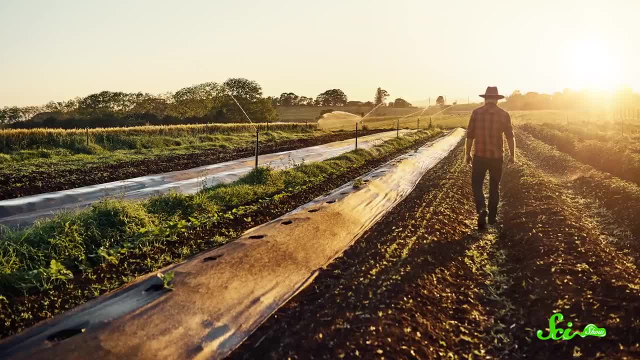 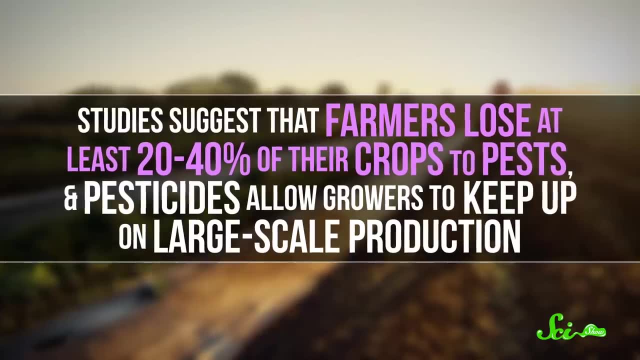 And let's face it, pesticides make growing food more cost-effective. Studies suggest that farmers lose at least 20 to 40 percent of their crops to pests, And pesticides allow growers to keep up on large-scale production. That means food is cheaper. 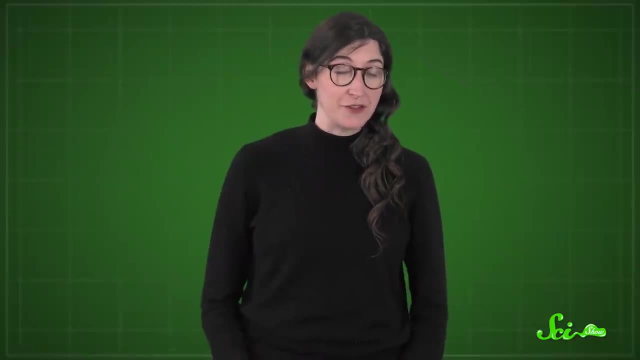 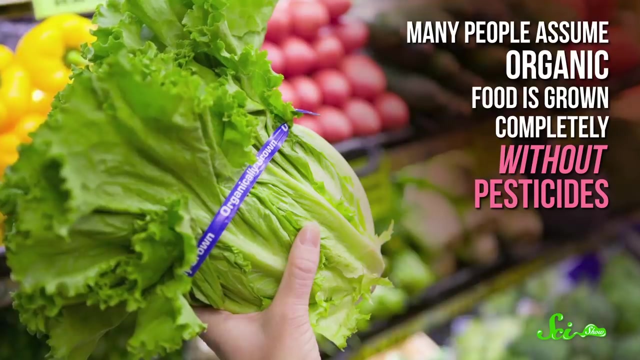 It doesn't just apply to regular produce either. It also applies to the fancy organic stuff. Many people assume organic food, at least as it's legally defined in the US, is not organic. Organic pests are grown completely without pesticides, But that's not true. 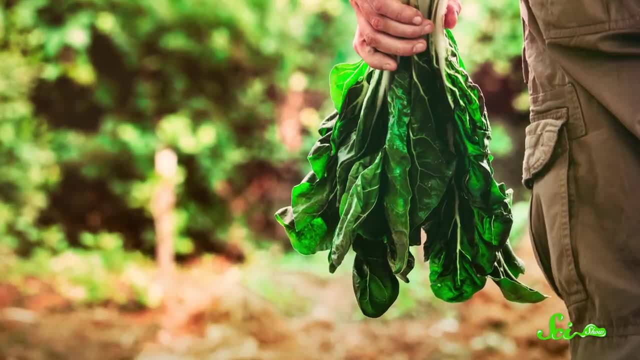 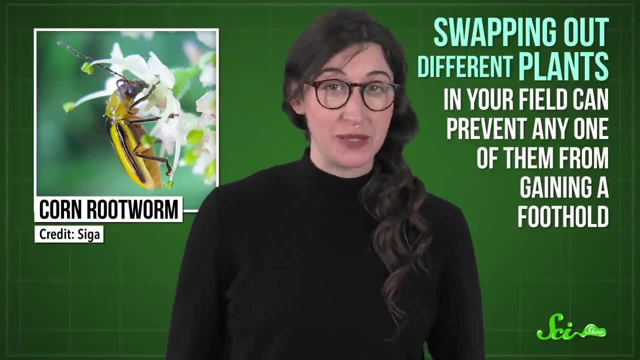 Organic farmers are supposed to do everything they can to avoid using pesticides in the first place, like rotating which crops they grow, Because many pests only attack certain crops. swapping out different plants in your field can prevent any one of them from gaining a foothold. 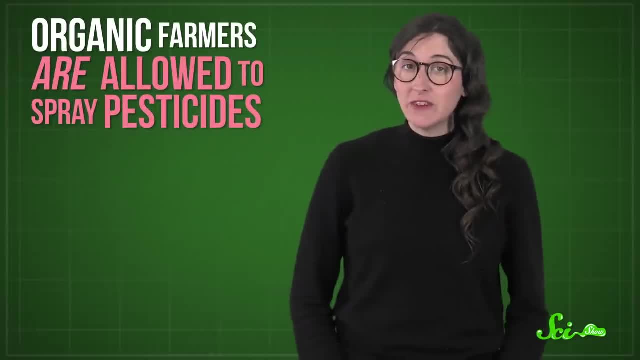 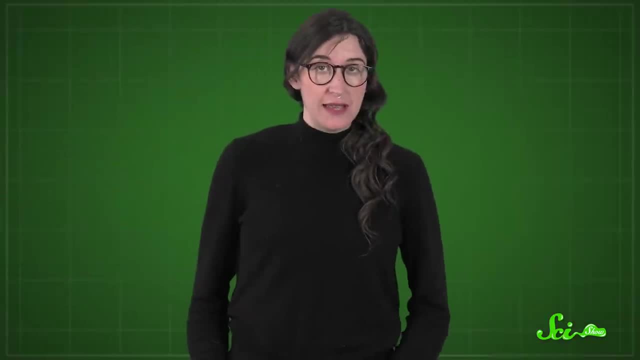 But if those methods fail — and often they do — organic farmers are allowed to spray pesticides. They just can't be man-made, although there are a few exceptions. Perhaps because of this And because people generally trust natural things over the ones humans cook up many 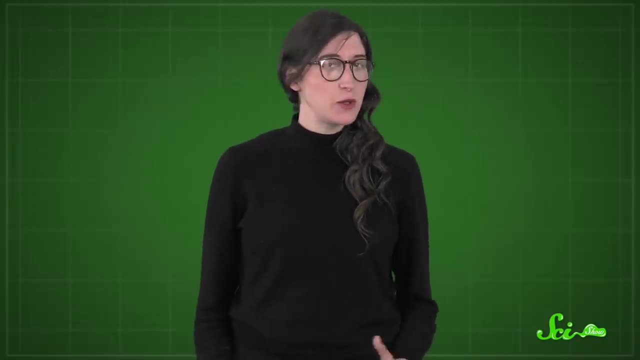 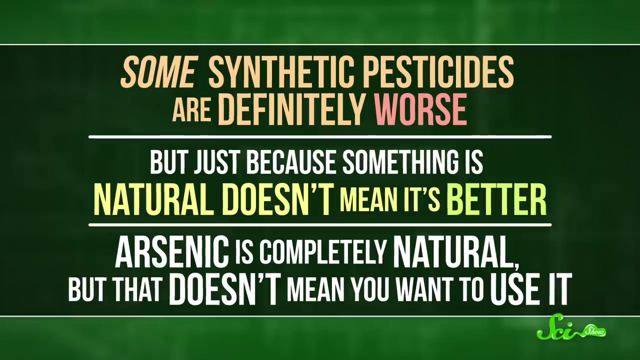 consumers have assumed that synthetic pesticides must be worse than natural ones, But that's only sometimes true. Some synthetic pesticides are definitely worse, But just because something is natural doesn't mean it's better. Arsenic, of course, is completely natural. 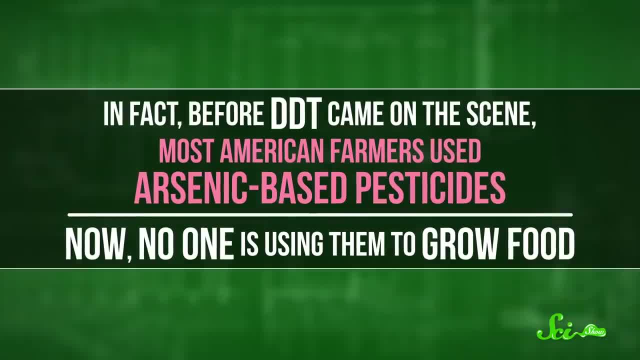 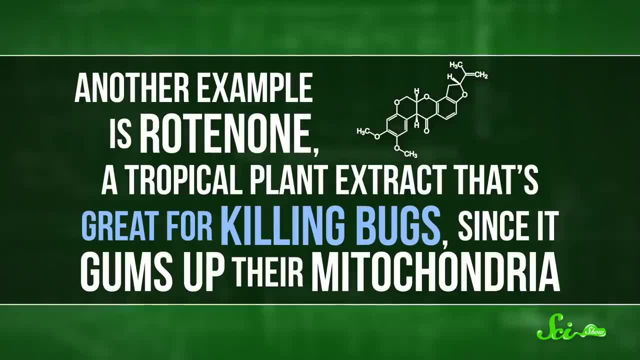 But that doesn't mean you'd want to use it. In fact, before DDT came on the scene, most American farmers used arsenic-based pesticides. Now, thankfully, no one is using them to grow food. Another example is rotenone, a tropical plant extract that's great for killing bugs, since 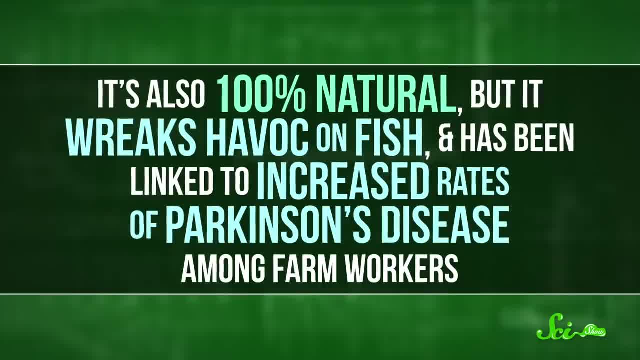 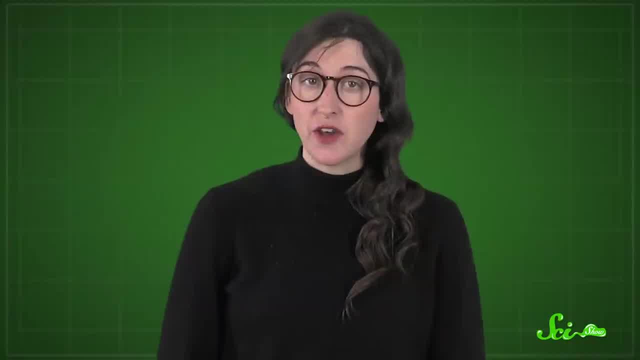 it gums up their mitochondria. It's also 100% natural, but it wreaks havoc on fish and has been linked to increased rates of Parkinson's disease among farm workers. Because of other regulations, American farmers can't use rotenone anymore. 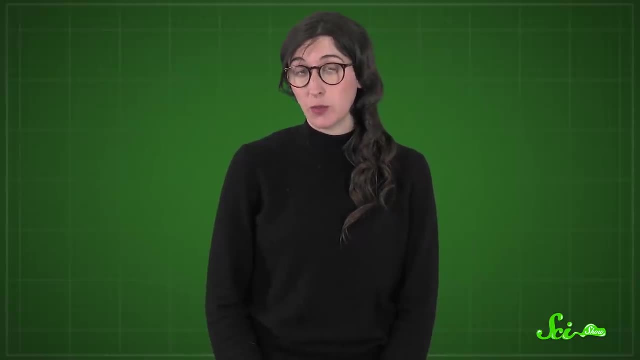 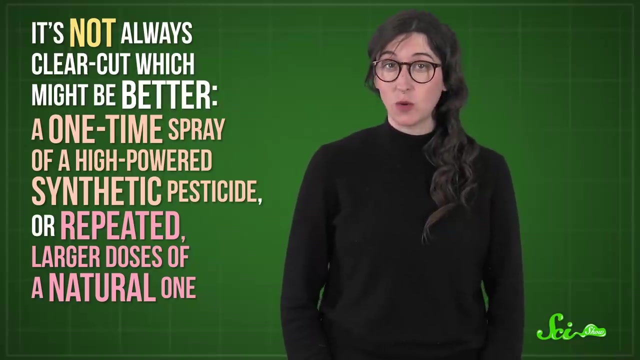 But at least right now it could still be on some imported organic produce. Dosage, as toxicologists are constantly reminding us, is also really important. Some scientists have pointed out it's not always clear-cut which might be better—a one-time spray of a high-powered synthetic pesticide or repeated, larger doses of a. 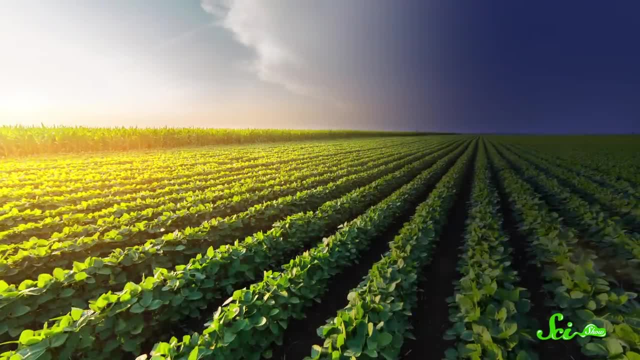 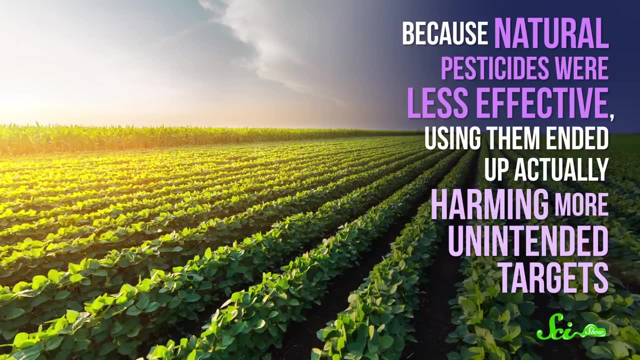 natural one. The research is still ongoing, but at least one study in soybeans found that, because natural pesticides were less effective, using them ended up actually harming more unintended targets. So the rules, then, are really rather arbitrary when it comes to synthetic versus natural. 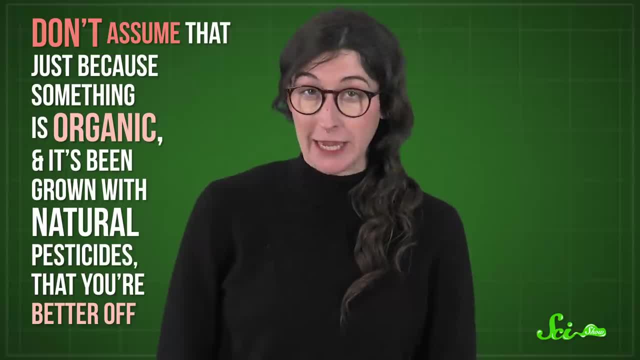 pesticides. Mostly, don't assume that just because a pesticide is toxic doesn't mean you should use it. But if you think that just because something is organic and it's been grown with natural pesticides that you're better off, it's not as clear-cut as you'd hope. Obviously, all of this isn't great for consumers, which includes all of us, because we all need to eat. But even though we're still working out the kinks with modern pesticides, you don't need to go and toss out all of your produce or anything. 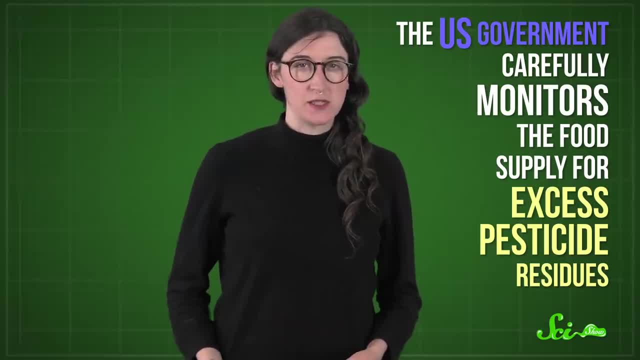 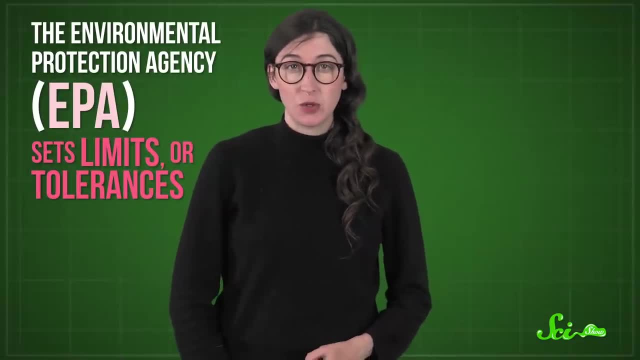 The US government carefully monitors the food supply for excess pesticide residues, so even if some make it into your groceries, you're going to be fine. The Environmental Protection Agency, or EPA, is the only agency that's going to be able to monitor the food supply for excess pesticide residues. 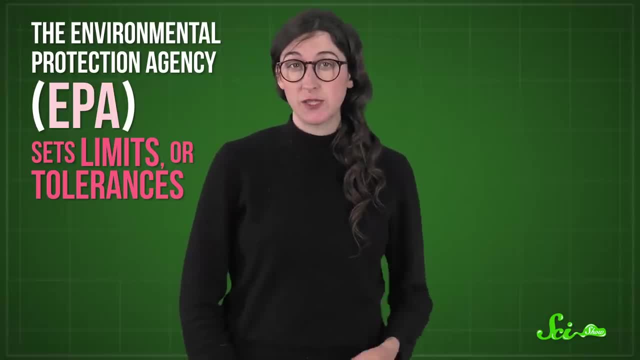 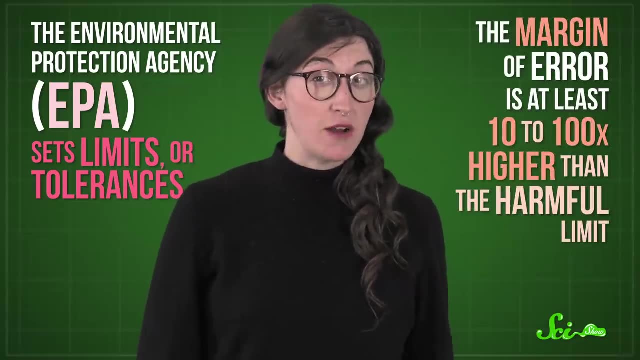 So even if some make it into your groceries, you're going to be fine. The Environmental Protection Agency, or EPA, sets limits or tolerances based on the available scientific data for the highest level of residue that's still safe. They also build in a margin of error that's at least 10 times, but often 100 times higher. 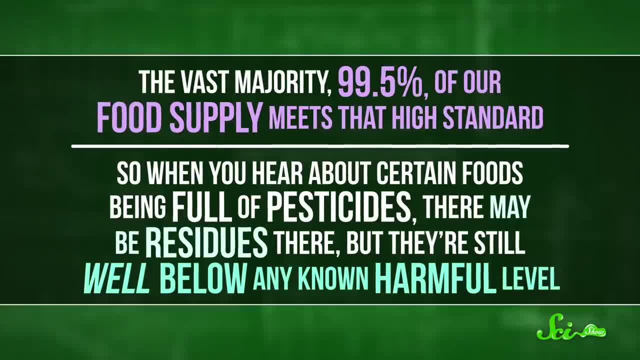 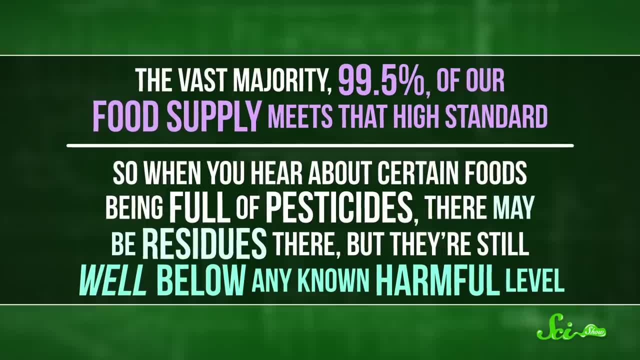 than what any study has suggested might be harmful, And the vast majority- 99.5%- of our food supply meets that high standard. So when you hear about certain foods being full of pesticides, there may be residues there, but they're still well below any known harmful level. Like for one pesticide, You'd have to eat more than 700 times the typical daily apple consumption to reach the EPA's already cautious tolerance level. Of course the monitoring program isn't perfect. It doesn't test all food for all pesticides and it also doesn't test for most organic. 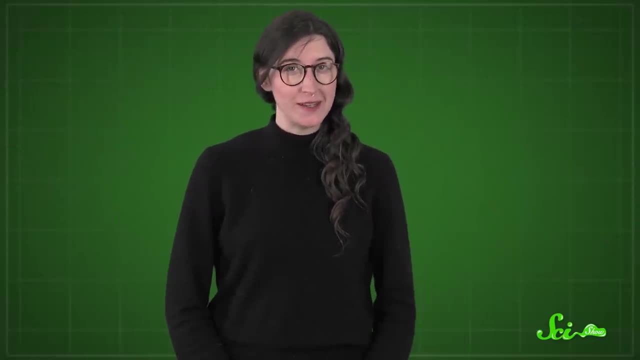 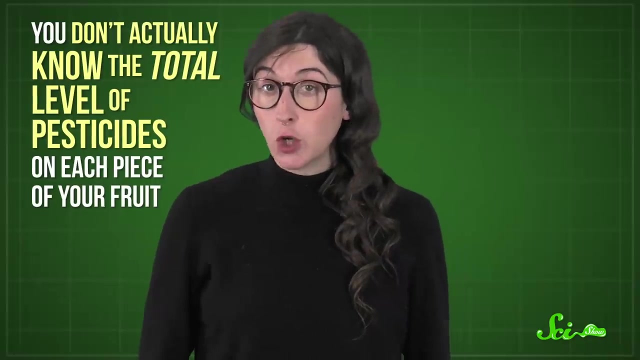 ones. That means comparing an organic apple to a conventional one isn't really fair. It's kind of like comparing apples to oranges, so to speak. Ultimately, this means you don't actually know the total level of pesticides on each piece of your fruit. 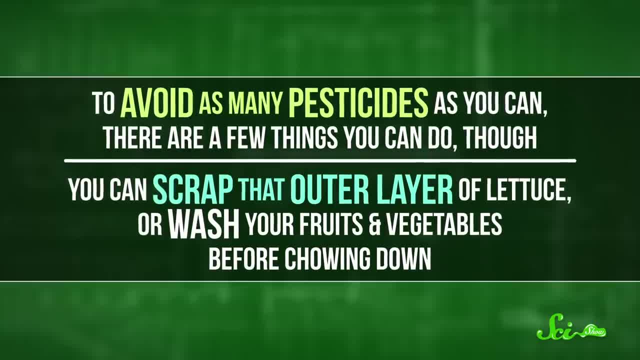 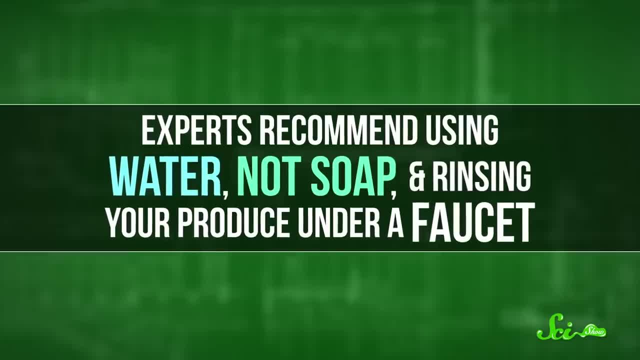 To avoid as many pesticides as you can. there are a few things you can do, though, Like you can scrap that outer layer of lettuce or wash your fruits and vegetables before chowing down. Experts recommend using water, not soap, and rinsing your produce under a faucet. 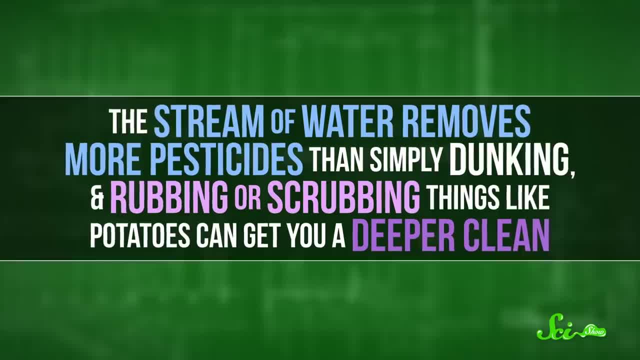 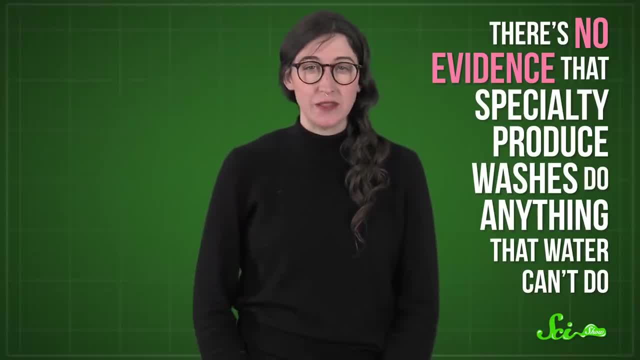 The stream of water removes more pesticides than simply dunking And rubbing or scrubbing. things like potatoes can get you a deeper clean. There's no evidence, though, that specialty produce washes do anything that water can't do. Washing won't remove every last molecule of pesticide. But it does help for most foods. You can also feel generally better about the pesticide situation these days, Even if things aren't perfect. farmers and scientists are much more aware of the dangers of them, And they've gotten better about using them more carefully. 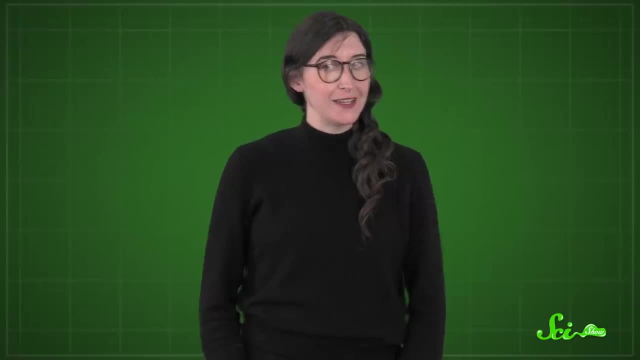 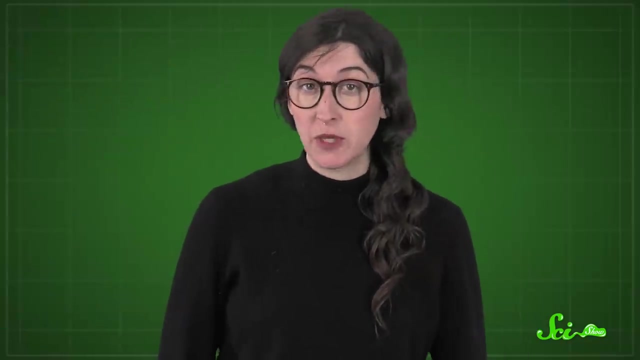 So, as much as people bemoan the good old days of agriculture compared with a half-century ago, people are ingesting fewer and less dangerous pesticides. Even the most famous ones people love to complain about aren't that bad. One of the most used and currently hated are pesticides: 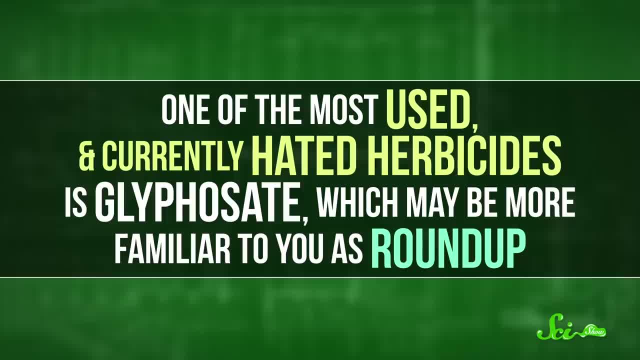 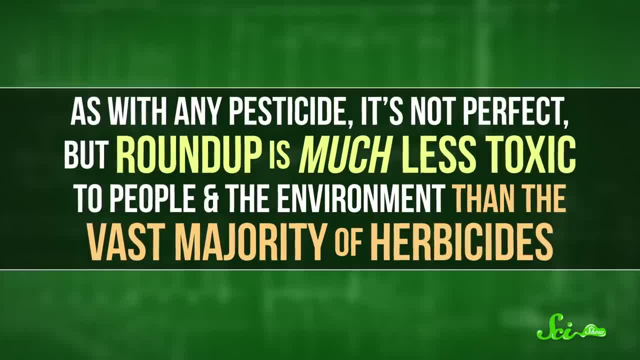 But they're not that bad. One of the most widely hated herbicides is glyphosate, which may be more familiar to you as Roundup. As with any pesticide, it's not perfect, But Roundup is much less toxic to people and the environment than the vast majority of. 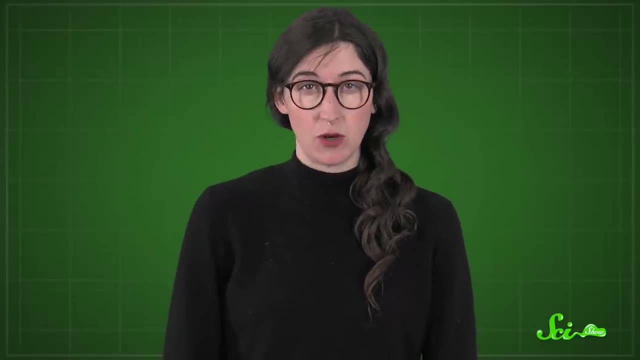 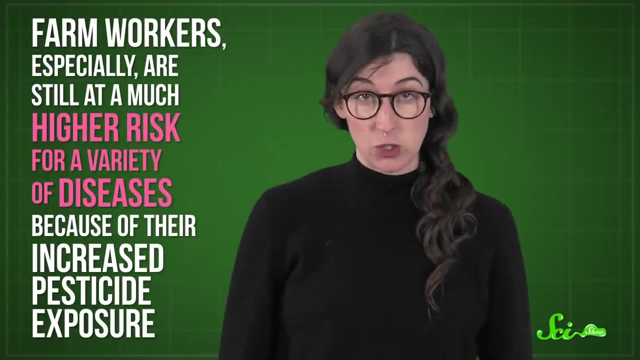 herbicides, You don't want to sit down to a dinner plate full of it, but all things considered it's not the worst thing out there. Of course, that's not to say the situation is ideal either. Farmworkers, especially, are still at a much higher risk for a variety of diseases, because 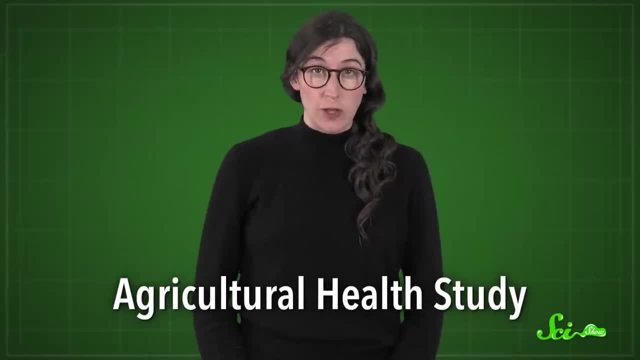 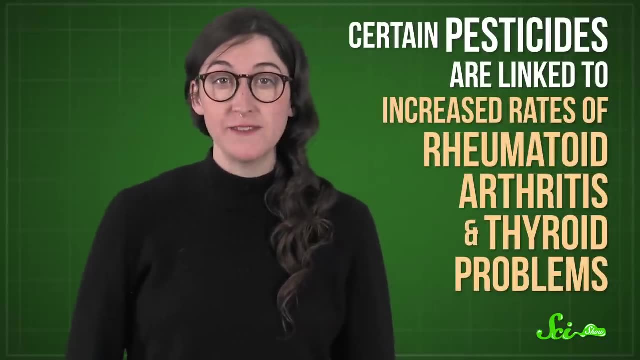 of their increased pesticide exposure. The long-running agricultural health study has shown that pesticides are not the worst. They're not the worst. The World Health Study has been tracking the health of people who apply pesticides for a living for 25 years. It's found that certain pesticides are linked to increased rates of rheumatoid arthritis. 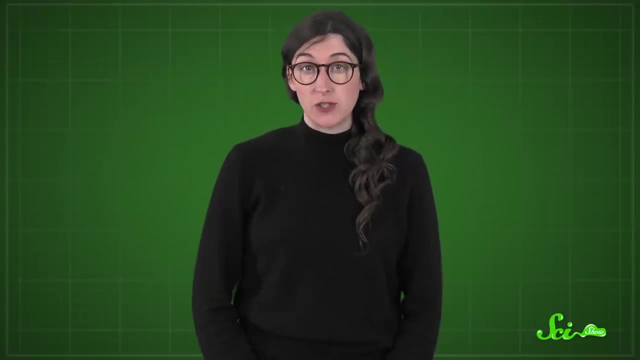 and thyroid problems, But in general, awareness about the possible dangers of these chemicals to people and the planet means we're less likely to indiscriminately use something like DDT before learning more about it. Scientists, too, are working on coming up with new, less toxic options for the future. 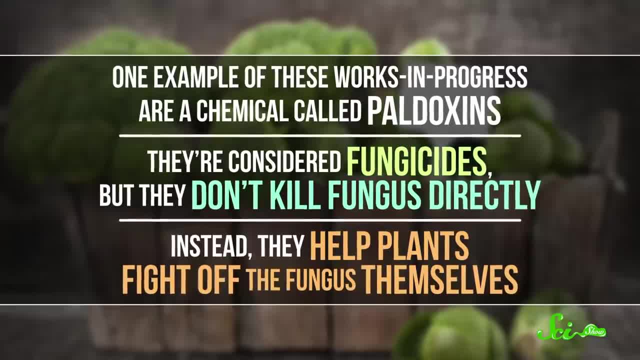 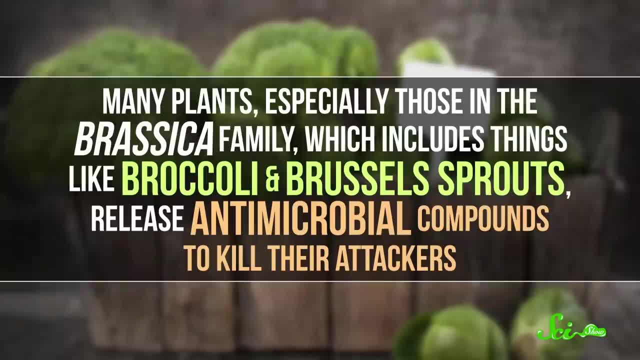 One example of these works in progress are a chemical called polyphenol. They're considered fungicides, but they don't kill fungus directly. Instead, they help plants fight off the fungus themselves. Many plants, especially those in the brassica family, which includes things like broccoli. 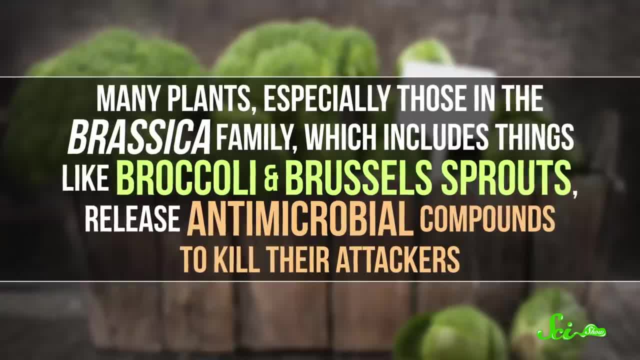 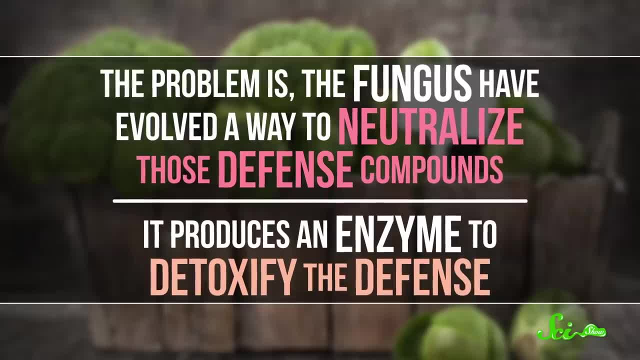 and brussels sprouts release antimicrobial compounds to kill their attackers. The problem is the fungus have evolved a way to neutralize those defense compounds. It produces an enzyme to detoxify the defense. The idea behind paldoxins is to remove that counterattack and destroy that fungal enzyme. 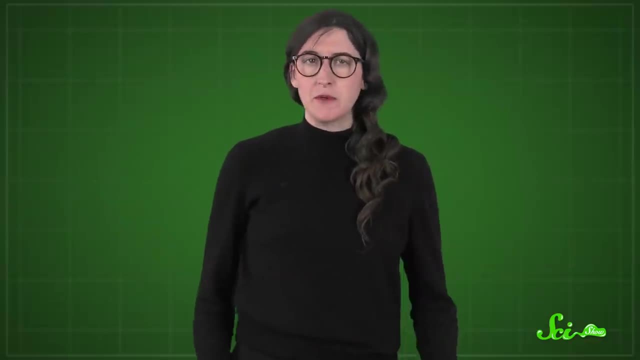 to make it easier for the crop to win the battle. It's kind of like fixing the match in favor of king broccoli. We don't know for sure how well these would work or how safe they would be, But because it's a very specific way of undermining a certain pest, biologists think